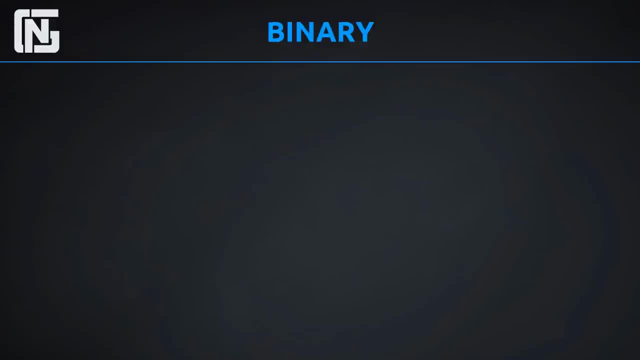 to IP addressing And to reinforce your understanding of binary ones and zeros. we need to know that a one or a zero is an on or an off. A one means on and a zero means off. A one means there is signal. A zero means there is no signal Right. Remember that. 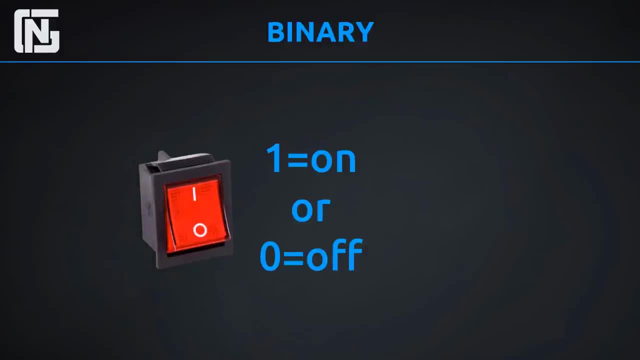 So this is probably something that you didn't know. Well, you may, but this is a cool little tidbit of information. If you look at a switch, like on the back of your computer, it may have a line and then a circle, As you can see here, on this particular switch we have 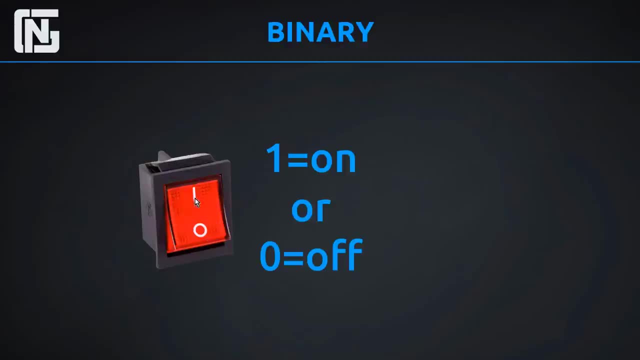 a line here and then a circle here. Well, this actually means on and off. This is a one and a zero. So if you turn this up, you're actually turning it on, And if you turn it down, this switch down- you're turning it off, because it's a one, meaning on and a zero. 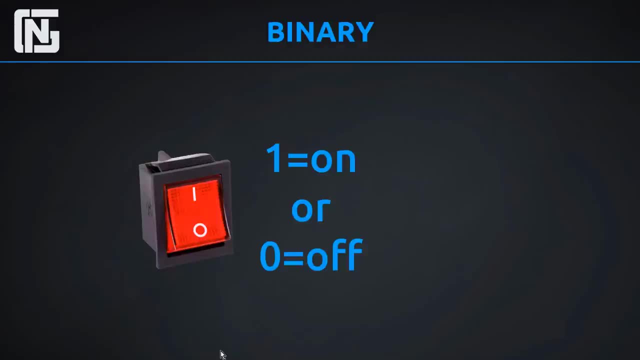 meaning off. That's kind of a cool tidbit of information. You've probably also seen this symbol before, And this is a power button to a computer, right? This also could be a power button to some other piece of electronics, But really this is a one with a zero You. 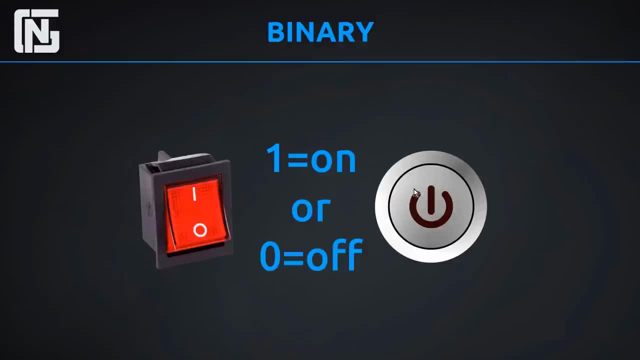 see it with a fully enclosed zero as well, But that's how this was configured, or that's how this was created- is to represent a one and a zero, which is on and off. That's why it's on a power button. Interesting fact, isn't it, guys? So that reinforces the fact. 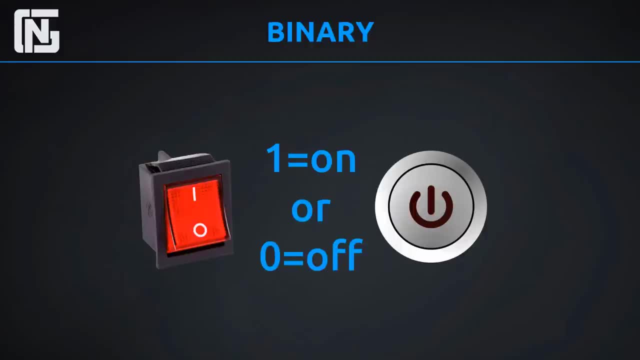 that we see binary. sometimes we don't even know it, and it means things and we don't even know it means something, And the basic form that a binary can tell you that it means something is an on or an off. All right, Let's move on, then and discuss what these ons and 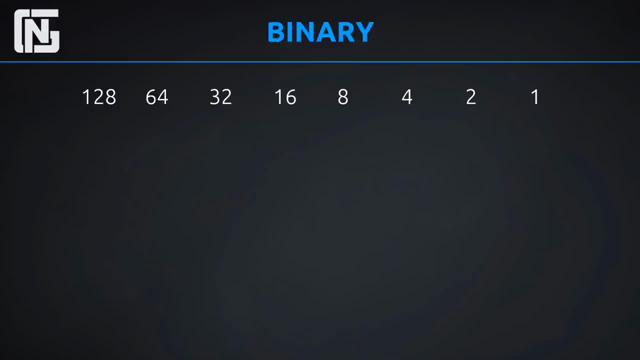 offs actually mean in more detail. So here we have something I'm going to call the most important chart for IP addressing and subnetting that you can ever create. That's my name for it. I'm not going to call it the golden chart or the fantabulous chart. I'm just going to call it the best chart you should. 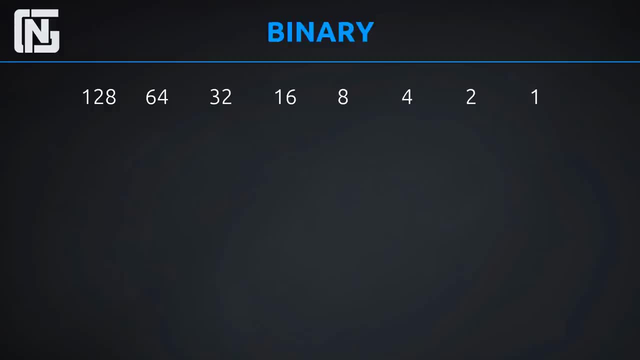 ever know for doing IP addressing and subnetting, because it really is. This is all you need to understand, or you need to understand how to manipulate these numbers here and how these numbers are created, And it's really actually easy. It's super easy, guys, And I'm just 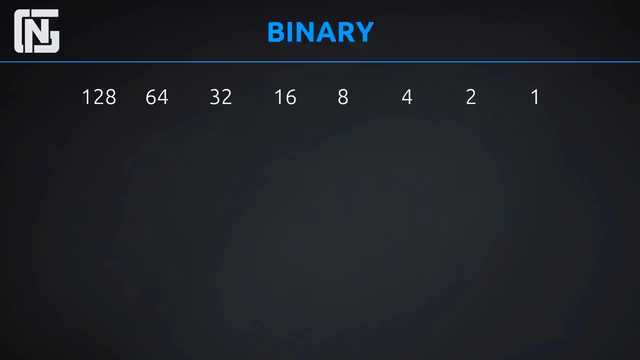 going to do a little bit of a rant here about subnetting and the fact that the way subnetting is taught these days- well, and actually the way it's been taught always- has been with using formulas as the primary method. You'll have all these different charts and these. 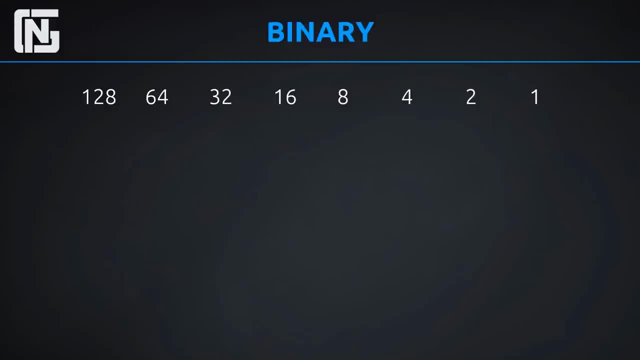 different formulas like 2 to the b minus 2.. Well, when we do our stuff, guys, it's all going to be just by binary. But understanding these numbers here we have on the screen is the way that we can make our lives so easy. 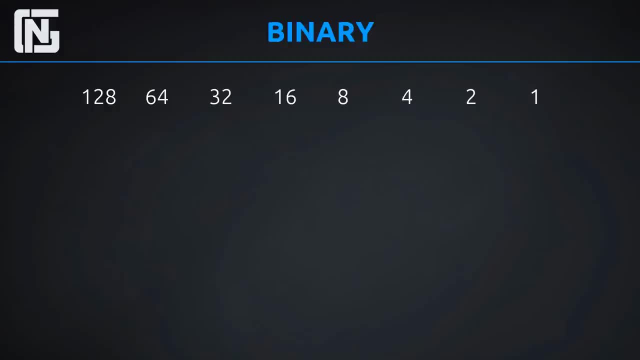 And when we get into subnetting- which we're not going to do in this lesson- but when you get into subnetting and you understand this, you're going to be able to do a lot of things. You're going to be able to do a lot of things. You're going to be able to do a lot of things. 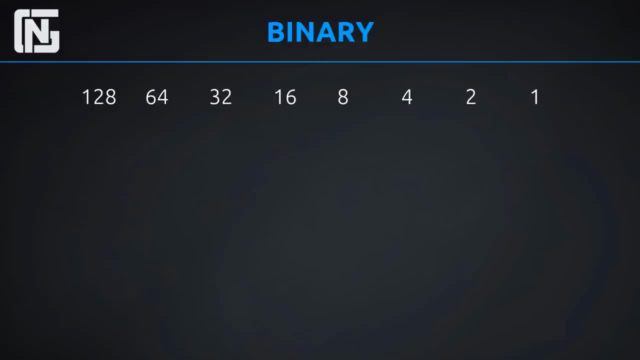 And when you understand this thing here, it's going to make your life so easy, guys, And you're really going to know what you're doing. It's going to bring everything together. If you've taken any subnetting classes before or you've done subnetting in the past and 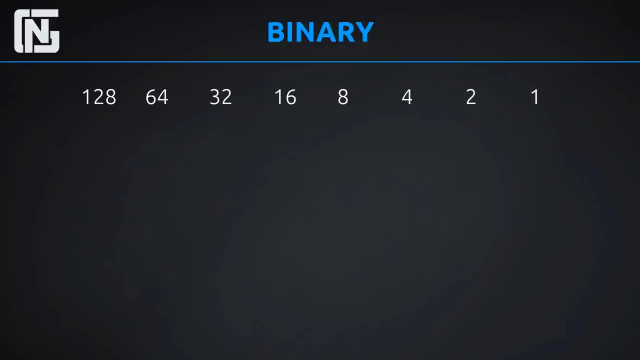 you've had a hard time. well, this is going to clear it up for you guys. I guarantee it. It's really great. So here we have our great chart right, And what this chart actually represents is binary values. So I'm going to put up on the screen some. 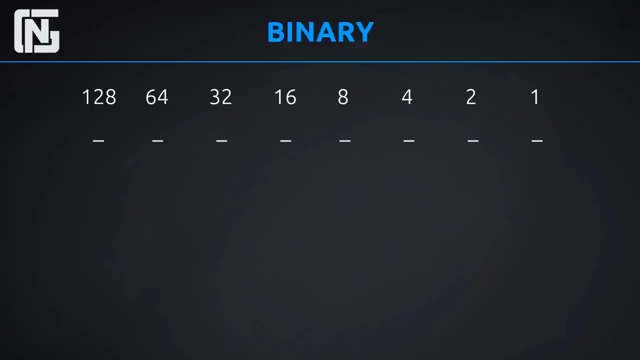 placeholders for some digits. Now, there's 8 placeholders here, meaning that there are eight binary digits, right? So we could fill these placeholders with either a zero or a one, and they would be representing if we're turning on or off these bit fields, right? And 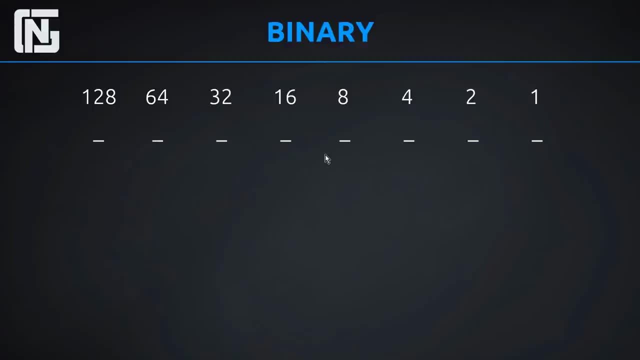 again, each one of these bit placeholders represents the number that's above it in the chart that we wrote, So let's go ahead and fill this with a series of ones and zeros. All right, we have some zeros and we have one one here, And I'm going to describe exactly what this calculates out to. 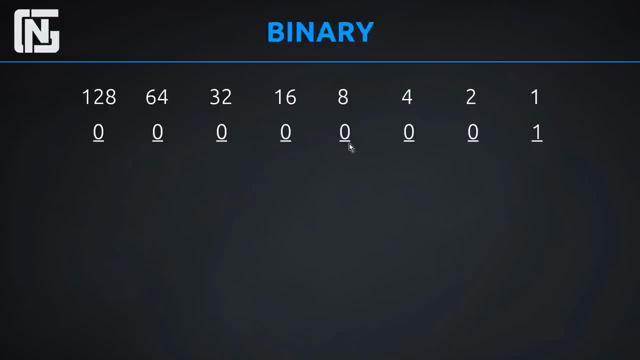 But before we do that, I want to make sure you understand that we're looking at eight binary digits And these eight binary digits together are considered to be an octet. So it's called an octet because oct means eight. So an octet is eight binary digits and an IP address and a network. 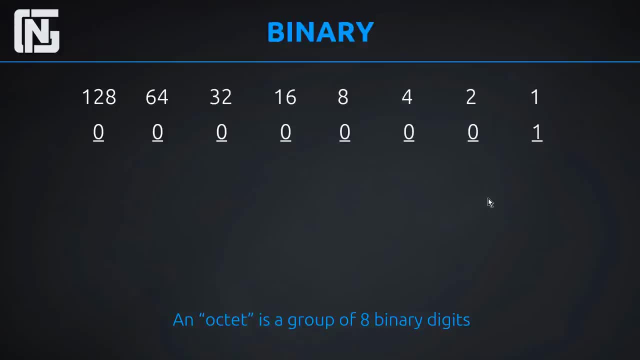 ID and a subnet mask. They're all made up of four separate octets, which are four separate groups of eight binary digits. If you multiply eight times four, that gives you 32.. So there's a total of 32.. 32 binary digits. But the point is we're looking at an octet here, right, And we are concerned with 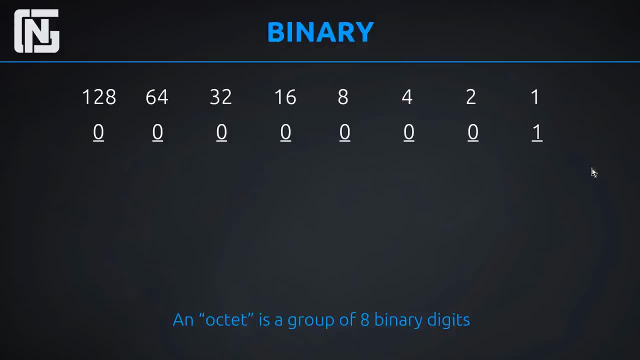 figuring out what this octet means. So each octet is built exactly the same way. Whether you're talking about an IP address, a network ID or a subnet mask, these bits to reference are always exactly the same. Starting at the right in the octet, it goes from one, then two, then four. 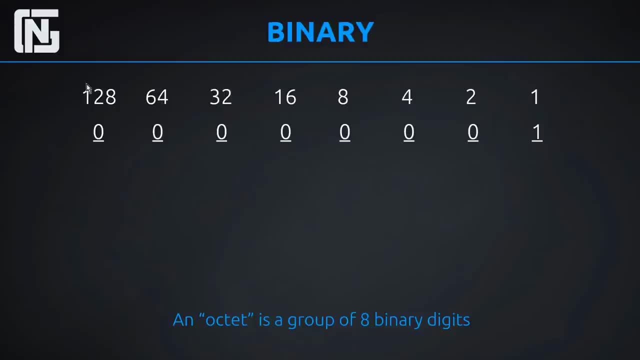 then eight, then 16,, 32,, 64,, 128.. All right, So that's how it works in the single octet. So now on to figuring out what this actually means. We said a binary can be an on, on and off. 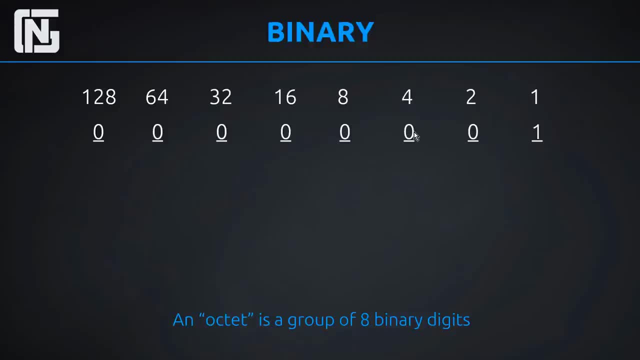 And that's why we represent it with a one or a zero. So anywhere we have a zero, we're saying that this bit field is actually turned off or this bit is turned off. So 128 is turned off in this example, 64 is turned off, 32 is turned off, All the way to two is turned off. The only thing 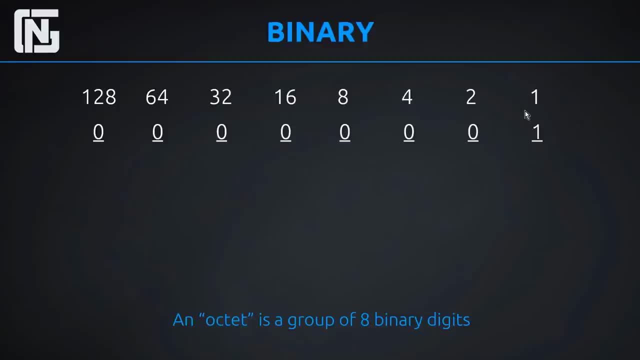 here that's turned on is the bit that is represented by the number one right. So when this is turned on, one right. So this means that this entire octet turns from binary into a decimal. one Makes sense If we added this one or if we turned on. let's say we turned on the field under the 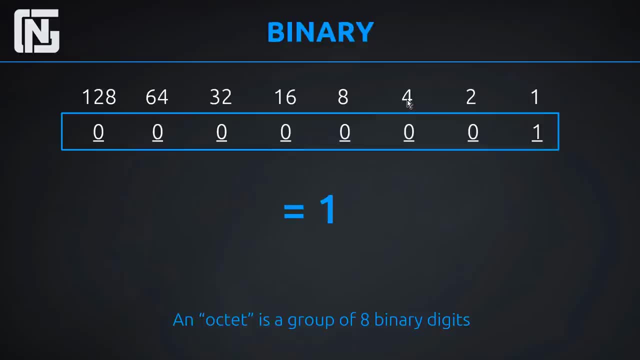 four. it would actually then be a five right, Because the four will be turned on and the one would be turned on, So that would be four plus one, equaling five. If these were all offs, then it would be a zero. All right, Let's do some more of these. 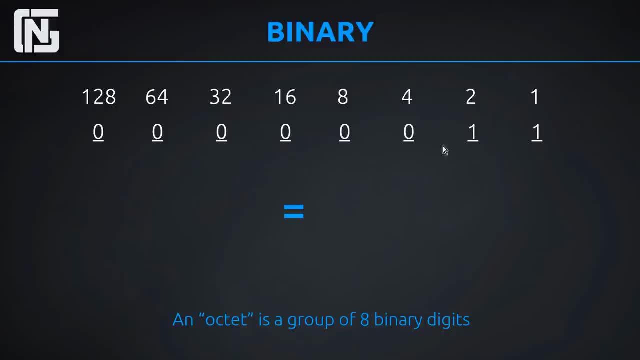 And put up another series of zeros and ones and see what that writes out to. All right, So now we have cleared out as well, everything from 128 to four Cleared out, meaning it's all zeros, But we have the two and the one turned on. So, with the two and the one turned on, what does that mean? 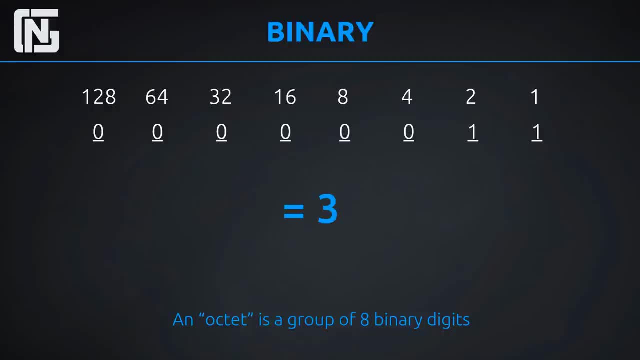 We have two plus one right, And that equals three. That's pretty easy. Let's look at another one. Let's look at this one here where we have the 32 field turned on and also the one, So 32 plus. 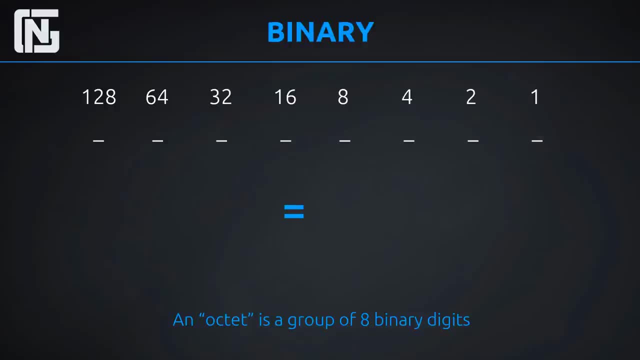 33.. I knew you guys could get that one. All right, Let's look at another one. Here we have only the 128 bit value turned on. So what does that mean, guys? That means our decimal value is 128.. Well, let's look at another interesting one. Next we're going to turn on all the bit. 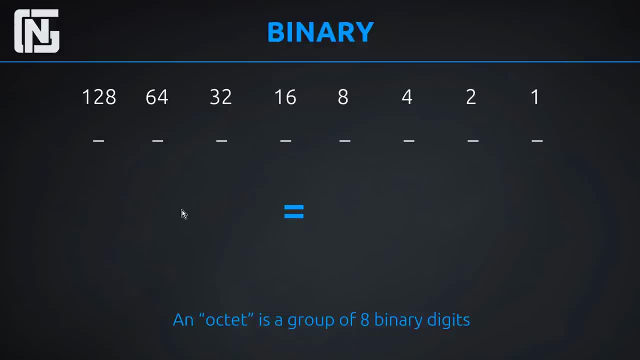 values after 128 and see what that adds up to. Here we have all the bit values after 128 turned on, So to figure out what this is, we could add 64 plus one. So we're going to turn on the 32 plus 16 plus eight plus four plus two plus one And we would find out that that actually 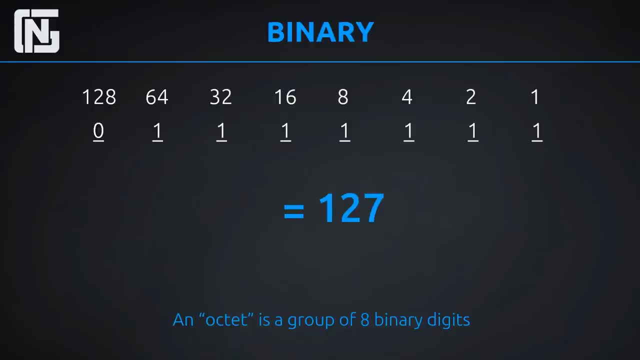 equals 127.. So what's so magic about this? Well, these adding up are always going to be one less than the number ahead of it, So we could already know that if all these were on that, they would equal 127, because this one less than this value here 128.. And let's say that we also had 64. 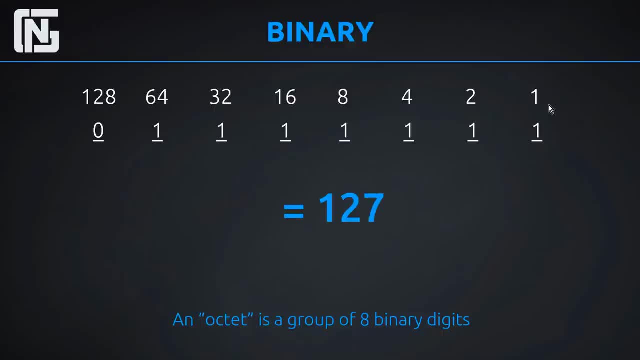 turned off right And we had just 32 and below turned on. Well, we'd know if we added those up 63. Does that make sense? I'm sure it does. Let's do that one more time. actually, Here we have one. 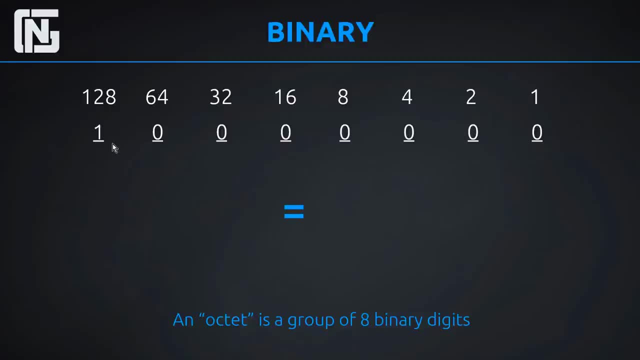 in the 128 field and everything else is turned off right. So that means that this octet turns from binary to decimal, meaning that it's 128 in decimal. Now, if we clear everything out and we just fill all these up with ones below 128, this binary, this 01111111 binary, translates into: 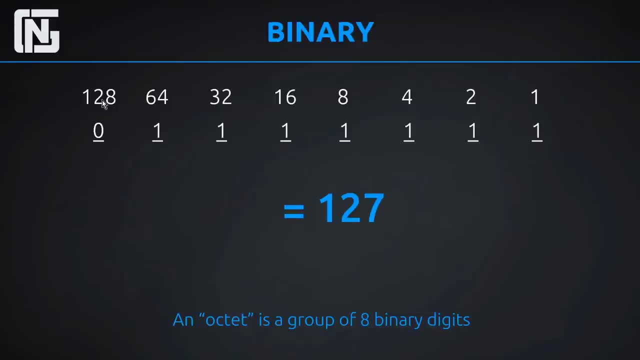 127, which is one less than 128.. The reason why I'm doubling down on this and telling you guys this twice is because we will utilize this to really super easily figure out things regarding subnetting in the future when we do our subnetting lesson. So I want you to get this point here. So that's. 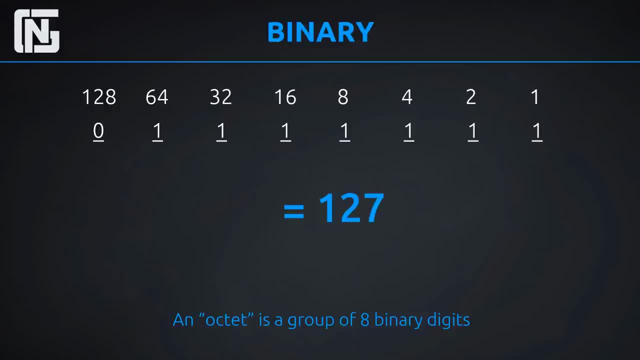 really how we dissect a octet. That's how we dissect eight binary bits and how we can change them into decimal format. So you could play around with this as much as you want. I do have some practice exercises. I'm going to start with this, but you can just figure out your own numbers Now if you add all of these. 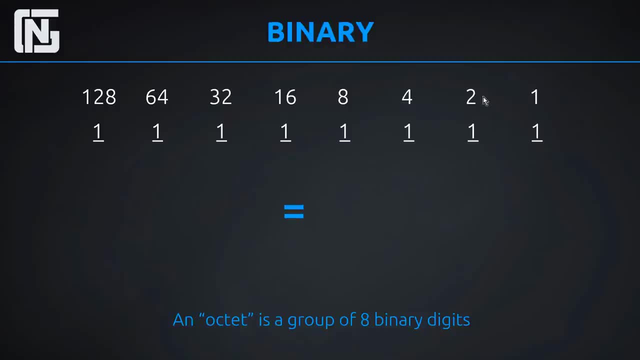 together. well, what does that make, guys? If we have all ones in these fields, what does that make? That makes 255, which is why you've seen this number before. When there's all ones in an octet, it equals 255. So you're never going to have a number higher than 255 in your IP address. 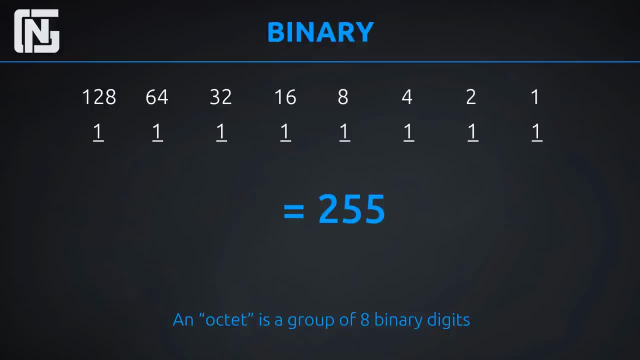 in your decimal IP address. You will never see a number higher than that. So you can think. if you want to get anything 255 or below, you could figure out what that would be in binary Right. So we can do this with eight bits. We can write in binary one all the way up to 255. 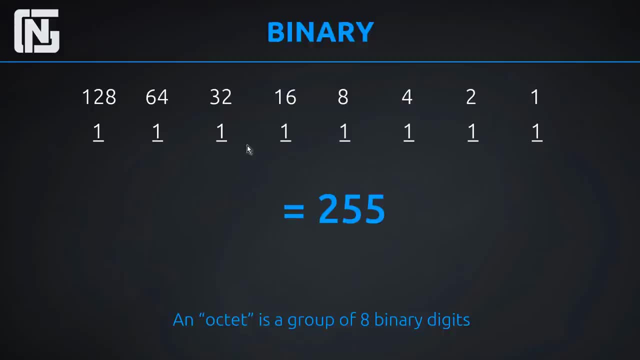 by changing these from different combinations of ones and zeros. Pretty cool stuff. If you haven't seen binary before, you can see how it's so useful. It's really awesome. All right, So let's go ahead and move on to our next exercise, guys, where we will look at an IP address in binary. So here we. 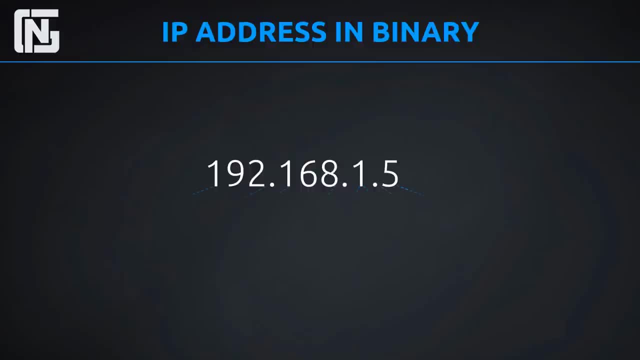 have an IP address: 192.168.1.5.. And if we break this out into binary, it'll look like this: We have four different octets, right, And we have four different sets of decimal numbers that translate to four different sets of binary digits, of eight binary digits, So it's eight here. 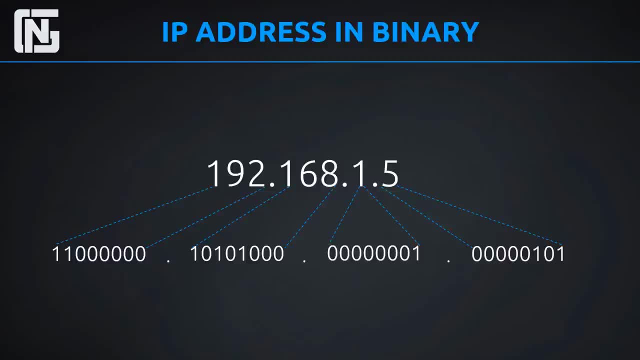 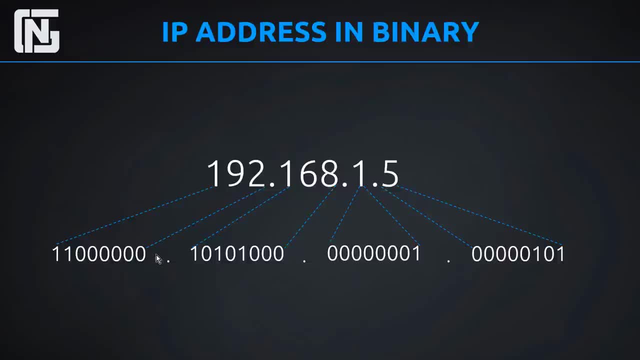 We could figure out what 1 is, what 5 is, And we could say, oh, that's how we came up with this binary octet, That's how we came up with this binary octet. Now, we could do that in our head if 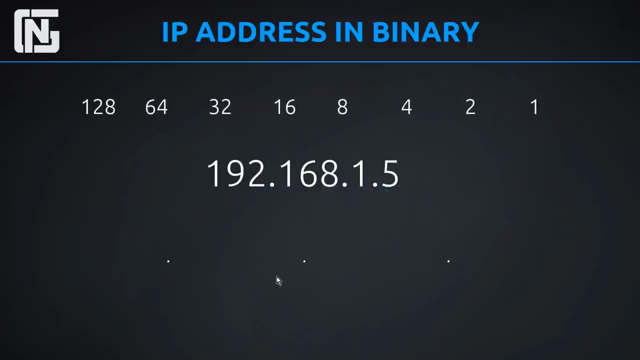 we want. But, guys, it's much easier if we use our awesome chart. So let's go ahead and use our awesome chart and do this again, or look at it by having our chart up, rather OK, So now we have 192, right, Well, 192,. we can look at our chart. Remember, this is eight. It's just eight digits. 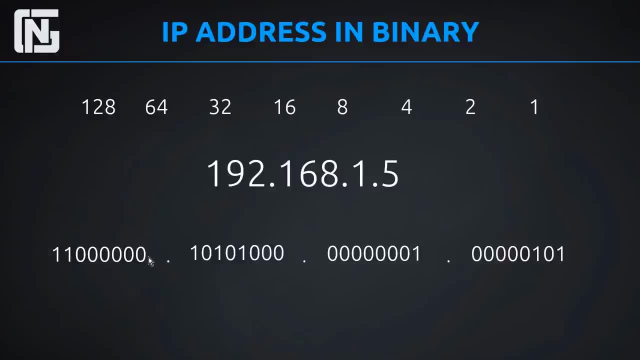 And let's look at the 192 decimal value. And if this was, if we didn't have this up here and we're just trying to figure it out- we would say, OK, what do we use in our chart to get to 192?? Well, we'll use the 128.. You always start out with the highest number in the chart. 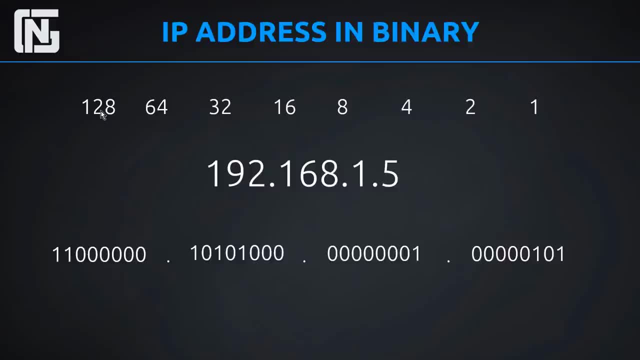 you can, which 192 includes 128,, right? So then you start adding things up, So we start with 128, and then we add 64 to 128. Well, 128 plus 64 actually equals 192.. So there we have it, We. 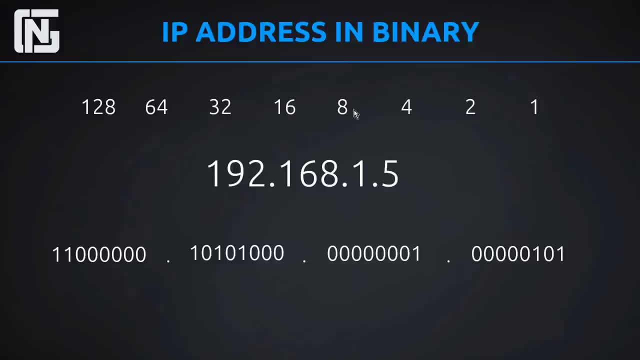 know that our binary will be 1, 1, and then 0, 0, 0,, 0, 0, 0, because we already got to 192.. Right, So we could write that down. Then, moving on to our second octet, here as it's called: